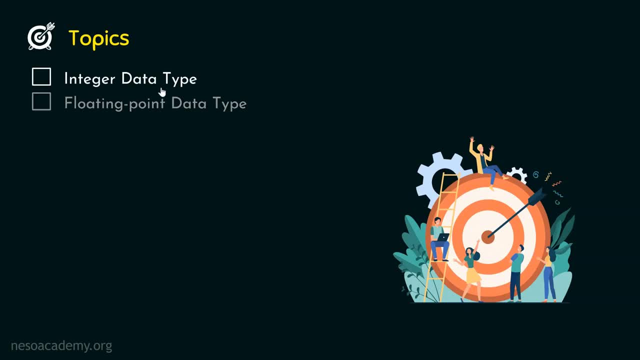 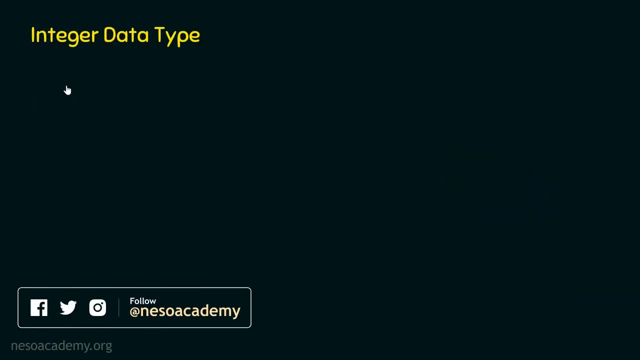 Let's first try to understand integer data type in Python. We can represent integers in Python. We already know that minus 1, 2, 0, 1, 5, 0, 0, 0, 3, 2, 3 are all examples of integers. 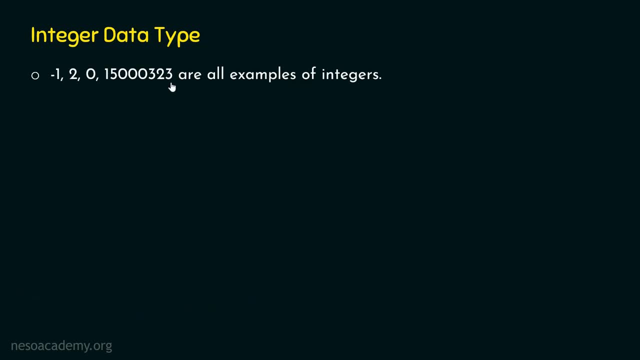 Thankfully, we can represent these integers in Python. We can even store them In Python. there is no limit on the size. We need to understand this: that Python puts no limit on the size of integers. We can have as long integers we want. 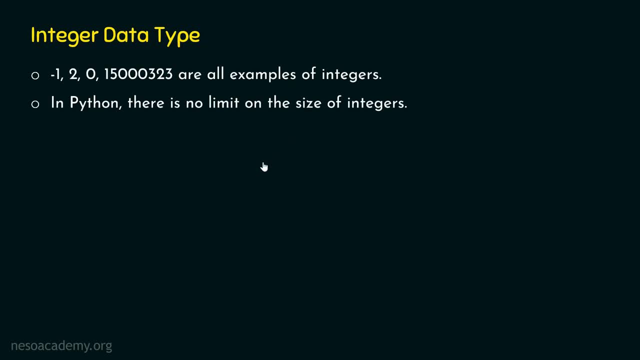 If you are an experienced programmer and if you already know C programming language, then you might know this already- that in C programming language we have a separate type to represent long integers or bigger size integers. We have long integers In Python. we have a separate type to represent long integers in C programming language. 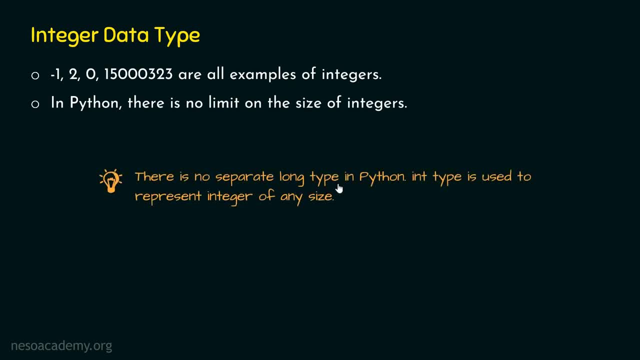 But in Python there is no separate long type, as it does not make any sense to have a separate long type. I have already told you that in Python there is no limit on the size of integers. This means we can have as long integers we want. 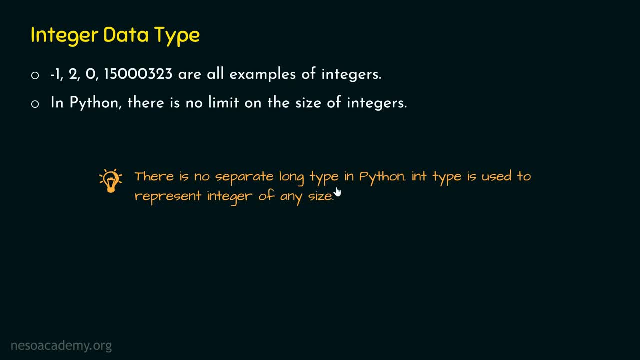 There is no need to have a separate type like long type in Python. Int type is used to represent integer of any size in Python. Also, you need to remember that in Python there is no need to explicitly specify the type. Python automatically understands the type of a value by seeing that value. 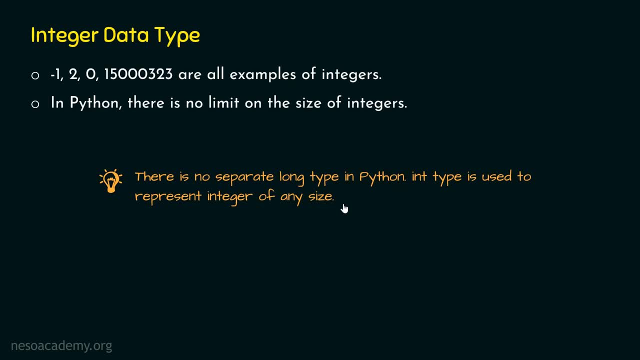 So we do not have to specify the type explicitly. Int type is used to represent integer of any size in Python. Now we know that we can represent integers in Python. We know that these are all decimal integers. This is how we say: minus 1, 2, 0, 1, 5, triple 0, 3, 2, 3.. 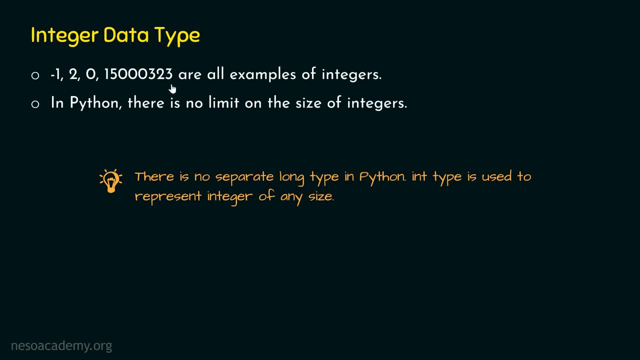 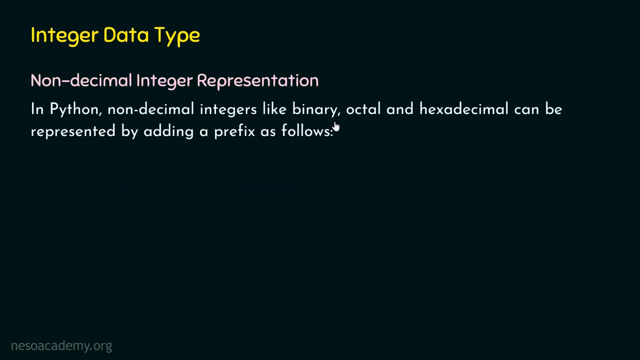 These are all examples of decimal integers. to be precise, Other than decimal integers, we can represent non-decimal integers as well in Python. Now we will try to understand How to represent non-decimal integers in Python. In Python, non-decimal integers like binary, octal and hexadecimal can be represented. 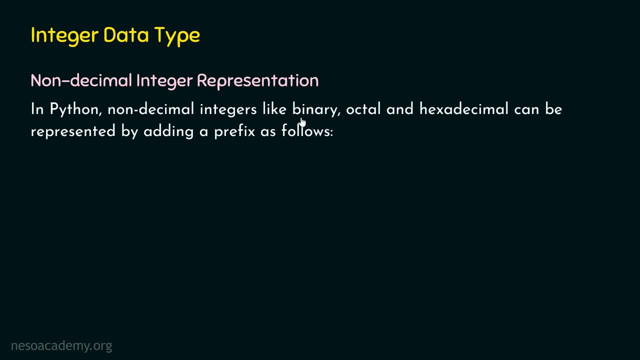 by adding a prefix as follows, We can represent binary, octal and hexadecimal numbers in Python. These are all non-decimal integers, as the base is not 10. for these integers, A binary number has base 2,, an octal number has base 8, and a hexadecimal number has base 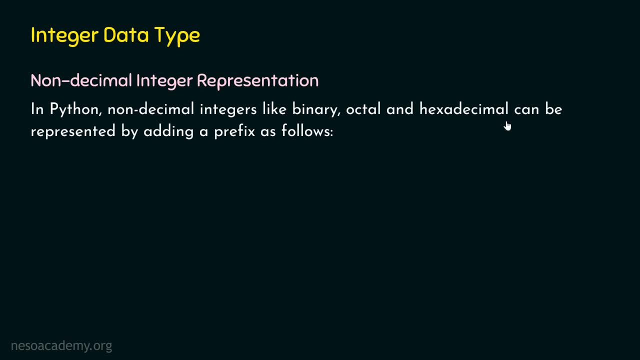 16.. Note that decimal numbers have base 10.. Okay, So these are all non-decimal integers. In order to represent these integers, we need to add special prefixes before them. Let's see what are all those prefixes. 0b or 0b can be used as a prefix to represent a binary number in Python. 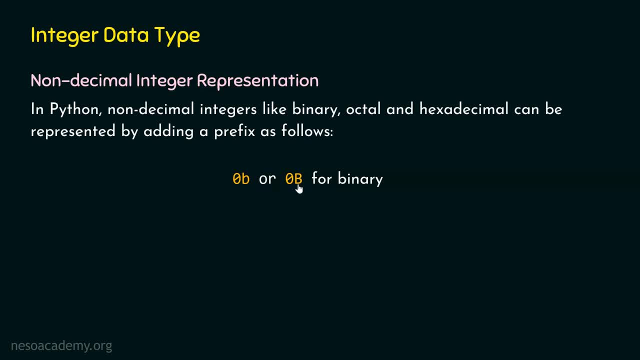 We can use 0b or 0b as a prefix in front of a number to tell Python that the number is a binary number. Similarly, we can use 0o or 0o for octal numbers. We can also use 0b or 0b as a prefix to represent a binary number in Python. 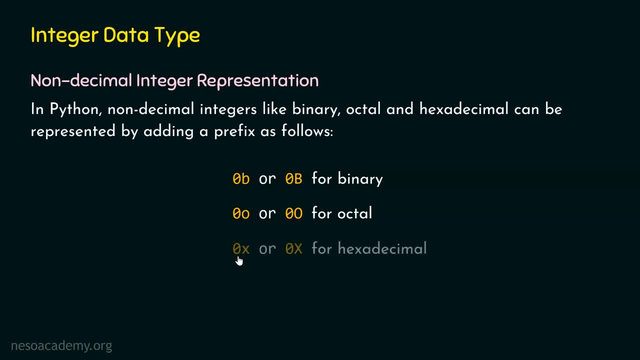 Similarly, we can use 0o or 0o for octal numbers. Let's see what are all these prefixes. We can use 0x or 0x for hexadecimal numbers, So we just need to add these prefixes before numbers to represent them as non-decimal integers. 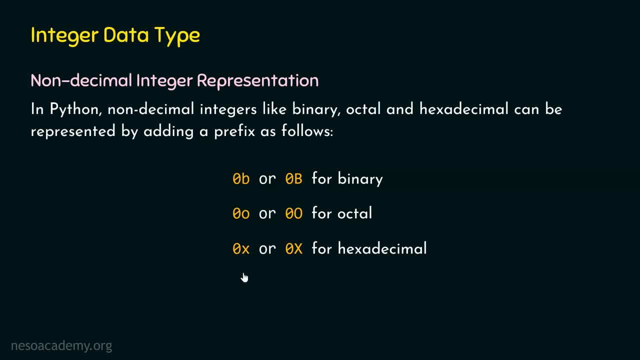 Now how to do this and what happens when we print them is what we need to understand. Note that, by default, when we try to print a non-decimal integer, the result will always be an integer. Now, if you don't know how to convert a non-decimal integer to a decimal integer, then it would. 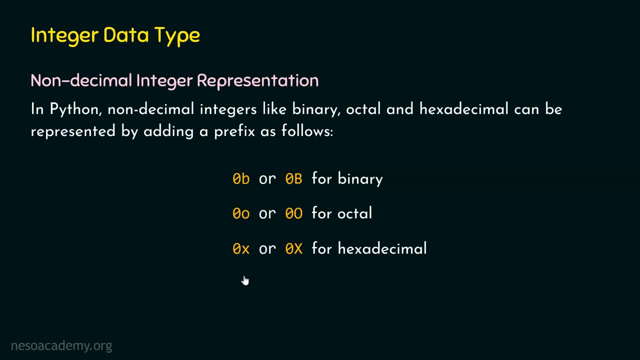 become difficult for you to interpret the result. You will get confused easily by seeing the result. So for this reason, we will now try to understand the complete process of how to convert a non-decimal integer to a decimal integer. Let's see how to do this. 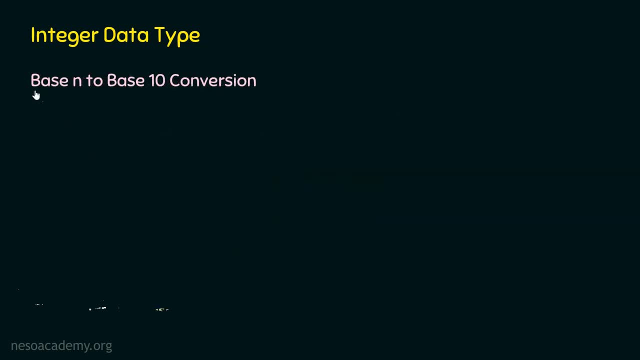 1. This means we will now learn how to convert base n to base 10 number. As I have already told you that base 10 represents a decimal number, Base 2, base 8, base 16 are used to represent binary, octal and hexadecimal numbers respectively. 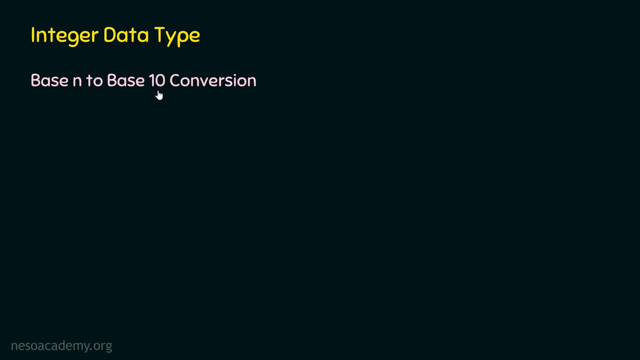 That is why I have written base n to base 10.. We can convert any base number to base 10 number. To convert a base n number to a base 10 number, each digit of the base n number needs to be multiplied from most significant digit to least significant digit, with n to the power. 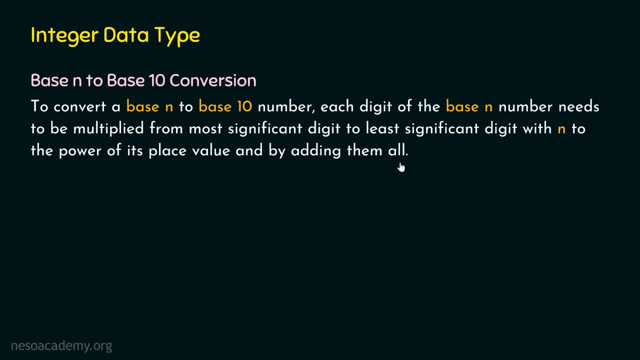 of its place value, and by adding them all. In order to understand this statement, we need to consider the following example: 2.. Let's say that we have this number, 1010.. Now, this is not a decimal number, because the base here is 2.. 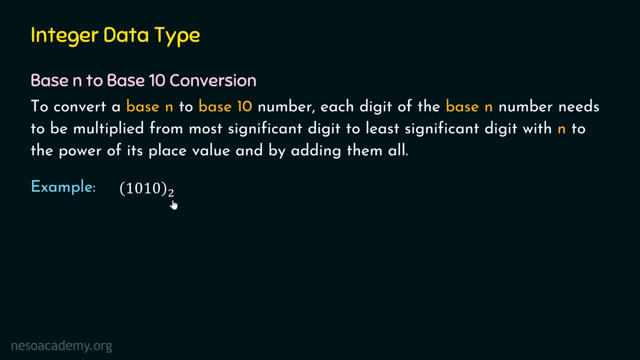 This means that this number is a binary number. This represents the base and this is our number. If there is no base, then by default it will be treated as a decimal number. But here we have this base 2,, which means that this number is a binary number. 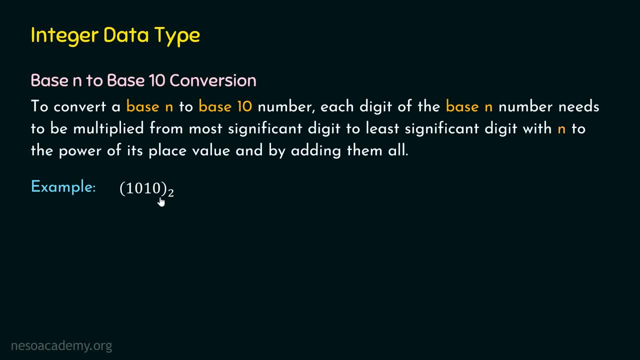 3. We need to convert this number to a base 10 number. This means that we need to convert this number to a decimal number. In order to convert this number to a decimal number, we need to multiply each digit of this number as what is written over here. 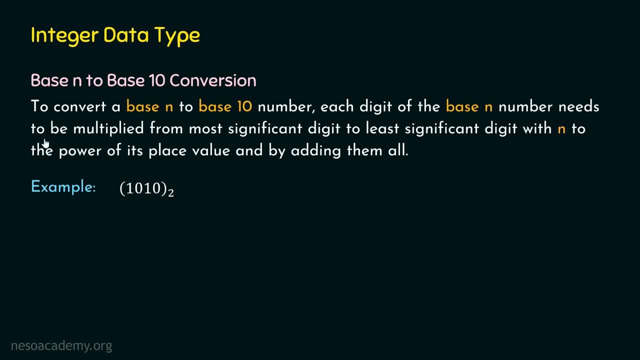 Each digit of the base n number needs to be multiplied from most significant digit. This means from this digit to least significant digit. So this is the base 10 number To least significant digit. this means up to this digit with n to the power of its place. 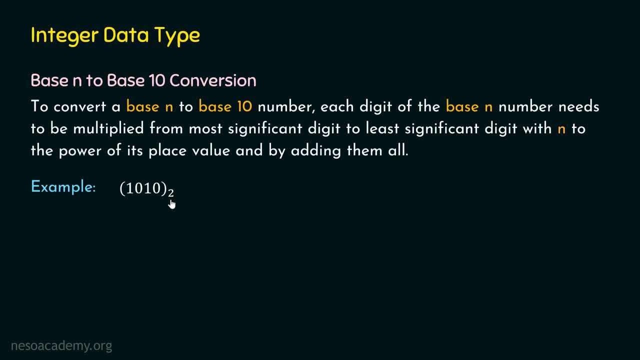 value. What is n here? n is 2.. We need to multiply each digit by n to the power of its place value. Place value of least significant digit is always 0 and from there the place value increases as we move left. So the place value of this digit is 0.. 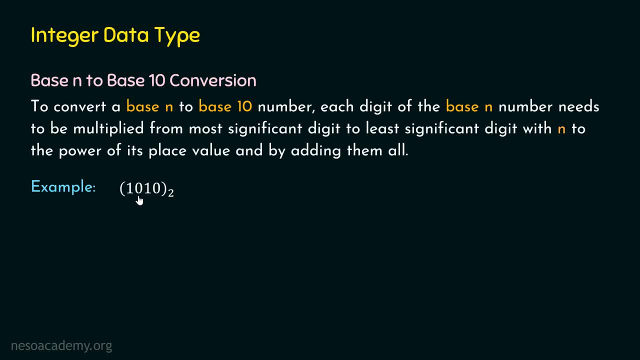 Place value of this digit is 1.. Place value of this digit is 2.. Place value of this digit is 3.. So the most significant digit has the place value 3.. We need to multiply each digit by 2 to the power of its place value. 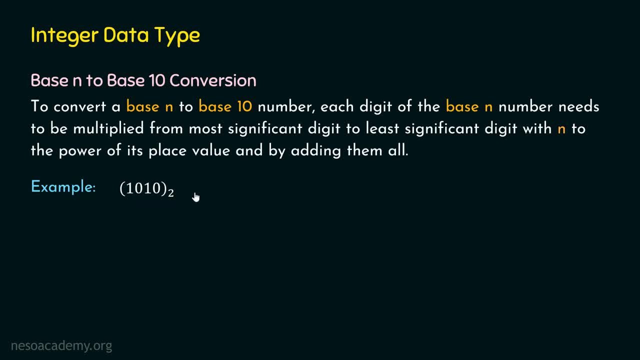 And then, finally, we need to add them all. This means that we need to multiply 1 by 2 to the power 3.. Then 2 to the power 2 must be multiplied by 0. This is what I have written. Then 2 to the power 1 must be multiplied by 1.. 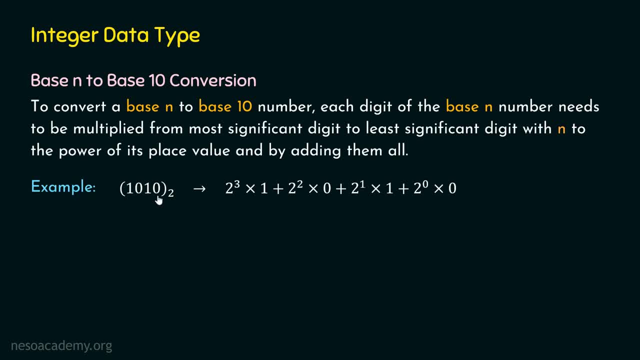 This is what I have written here. Then we need to multiply 2 to the power, 0 by 0.. This is what I have written here. Then, finally, we need to add all these terms. The result will be 10 base 10.. 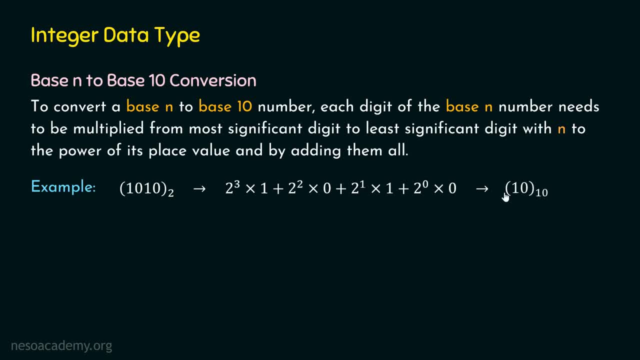 Note the base here. This is not a binary number, This is a decimal number. So this number is the decimal equivalent of this binary number, 1010.. I hope this process is now clear to you. Now let's consider one more example. 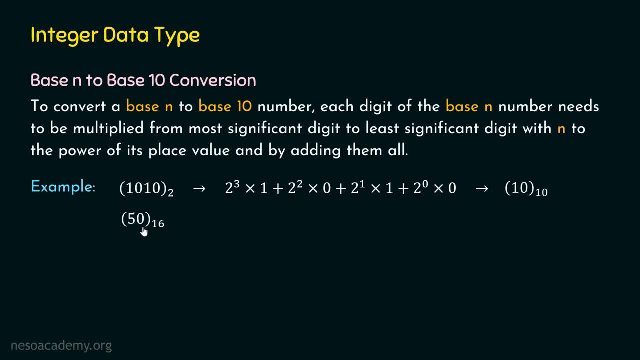 Let's say- this time we want to convert this number to a decimal number- This number is a hexadecimal number, as we can see this- that the base of this number is 16.. Now the process will be same. We need to multiply each digit of this number by 16, to the power of its place value. 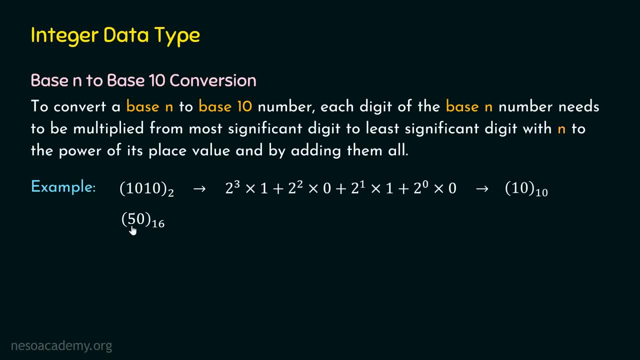 Place value of this digit is 0.. Place value of this digit is 1.. We need to multiply 5 by 16 to the power 1, and we need to multiply 0 by 16 to the power 0. And then we need to add them. 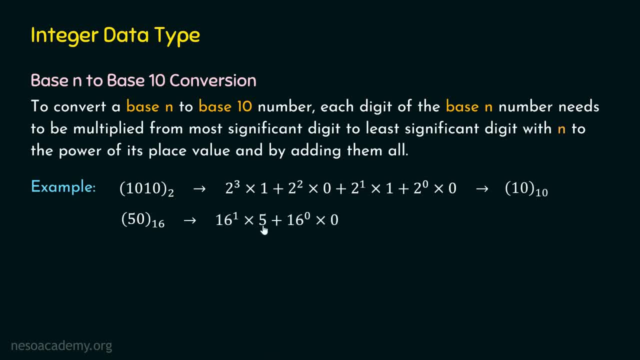 So we will get 16 to the power 0.. 16 to the power 1 into 5, plus 16 to the power 0 into 0, which is equal to 80.. This is the equivalent decimal number of this number. So in Python, if we try to print this hexadecimal number, we will get 80 as a result. 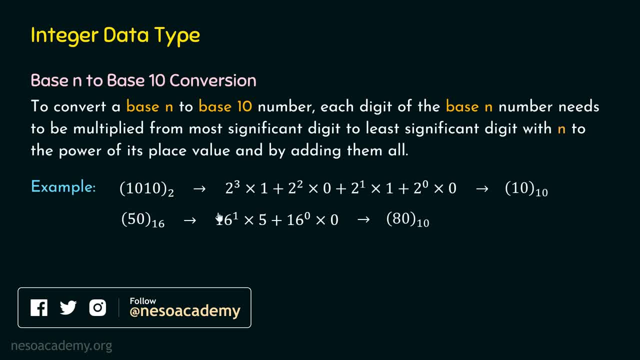 If we try to print this binary number in Python, we will get 10 as a result. As I have told you already, by default we will get decimal number as a result. Later we will understand that how to print the numbers. as it is. 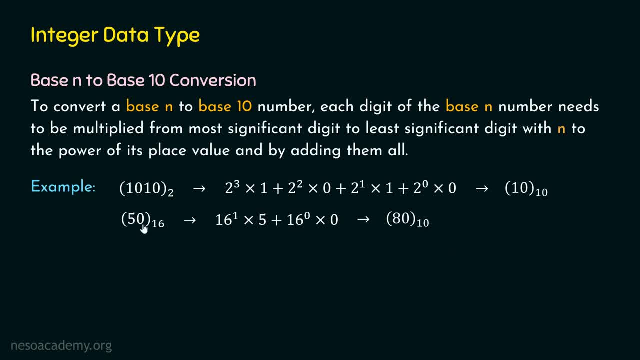 But right now you need to understand that if we try to print these numbers, we will get their equivalent decimal numbers. Okay, enough of theory. Let's try to print some non-decimal numbers on the screen and let's see what we will get. 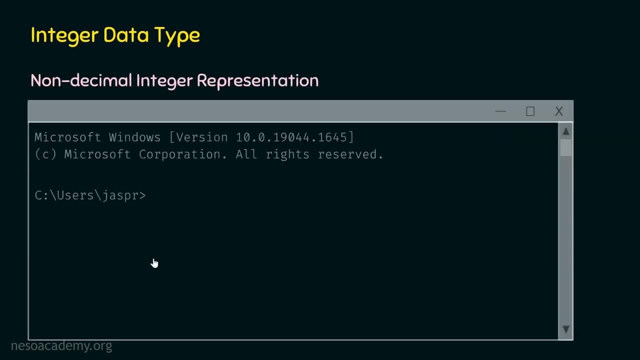 as a result. So we are in our command prompt. Let's type Python First. in order to activate Python interpreter, we need to type Python, and then we need to hit enter. We will get these three arrows. This means that interpreter is now active. 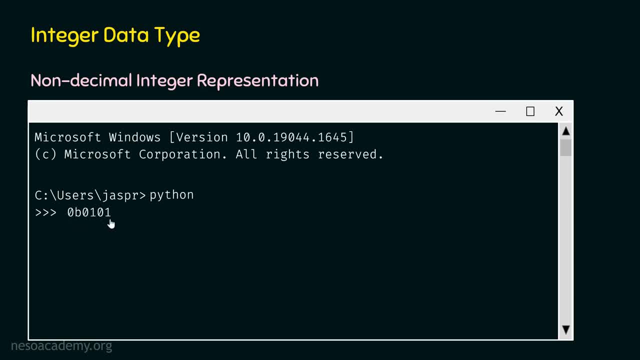 Now we need to type 0B0101.. As 0B is added before this number, this means that this number is a binary number. This is how we can represent binary numbers in Python. Then we know that interpreter will simply print the result. 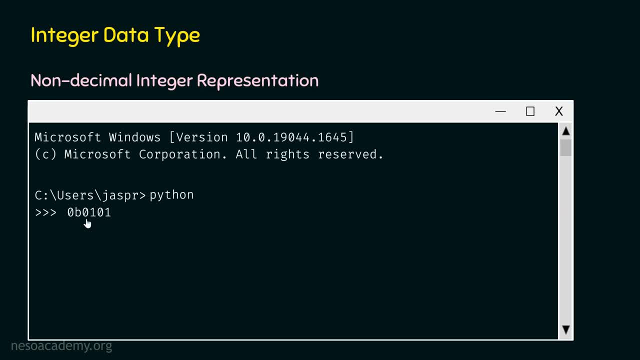 And we also know that we will get a decimal equivalent of this number. So when we hit enter, we will get this number 5.. Now this is homework for you, Why we are getting 5 here. You need to follow the same process of conversion of base n to base 10.. 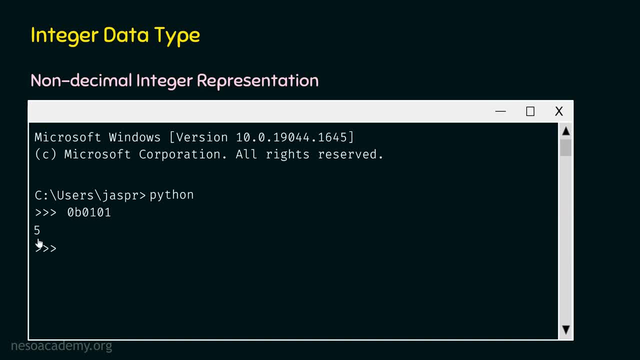 So do the same thing. Try to get this result Now. Interpreter is again active and now it is ready to receive the next command. Let's type 0072.. You can also write 0 capital O 72, and you can also write 0 capital B here. 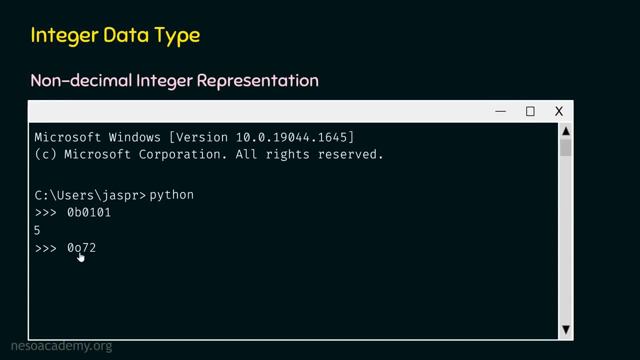 It doesn't really matter. Here I am writing 0 small o to represent an octal number. This is an octal number. This is not a decimal number. If we hit enter, we will get 58 as a result. That is why I told you it is important to understand base n to base 10 conversion, because 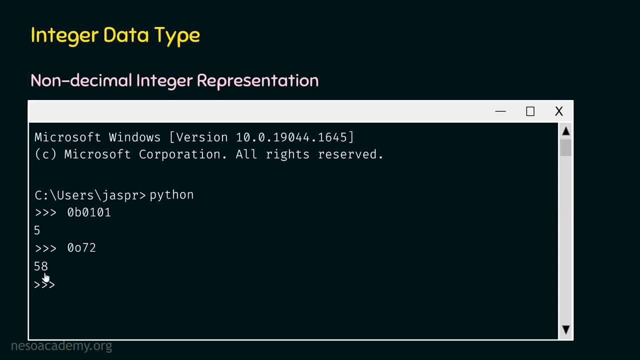 this result might confuse you. Again. we need to follow the same process of base n to base 10 conversion. This time the base is 8.. So we need to convert base 8 number to base 10 number. Now let's say we want to know what is the decimal equivalent of 0xff. 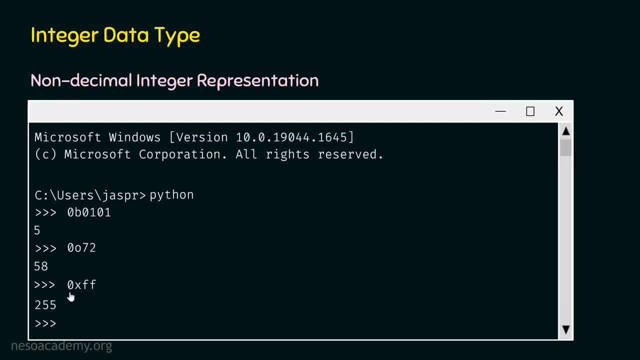 We will get 255 as a result. 0x is prefix for hexadecimal number. Note that in a hexadecimal number the digits are from 0 to 15.. 10 in hexadecimal is A. 11 in hexadecimal is B. 12 in hexadecimal is C. 13 in hexadecimal. 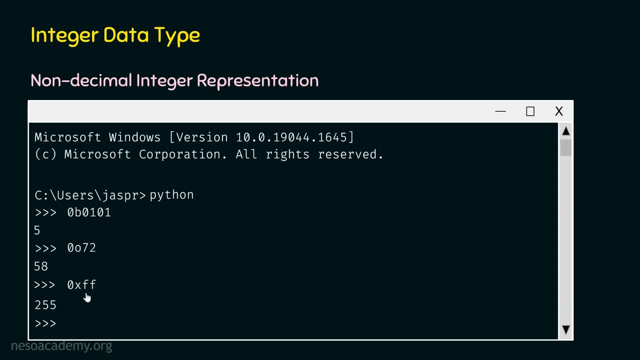 is D, 14 in hexadecimal is E and 15 in hexadecimal is F. So F is the decimal equivalent of 0x. 0x is prefix for hexadecimal number. F in hexadecimal is equal to 15.. So note: in this case we need to multiply 15 by 16 to the power 0, and we also need to: 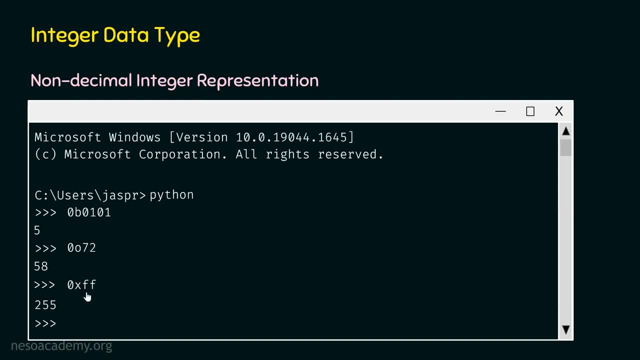 multiply 15 by 16 to the power 1 and need to add the results, So in this way we will get the equivalent decimal value of this number. This is how we can represent non-decimal integers, and now we know what happens when we print. 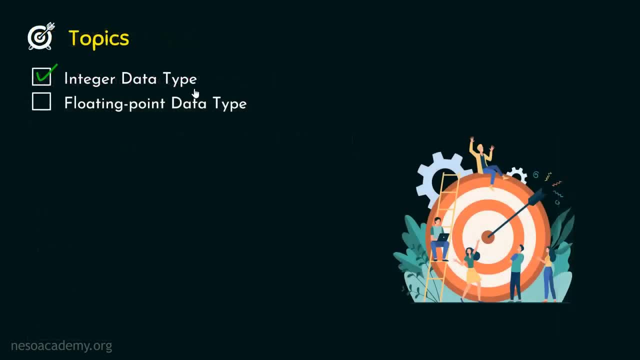 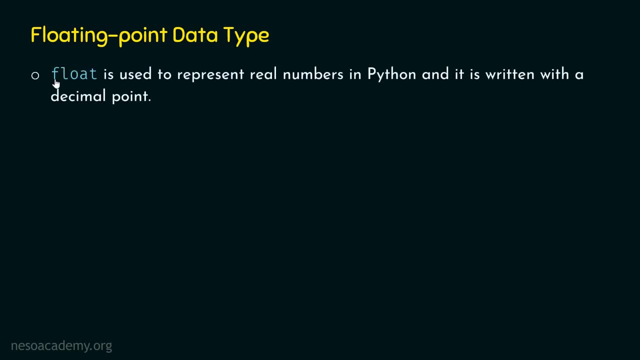 them. Okay, Let's start with integer data type. Now we are ready to understand floating point data type. Float in Python is used to represent real numbers and it is written with a decimal point. This is the difference between an integer and a floating point number. 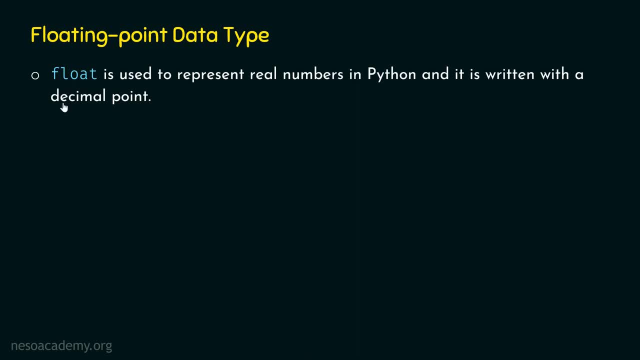 A floating point number is always written with a decimal point. These numbers are all real numbers. Okay, To specify the scientific notation: E or E. this means small e or capital E is added at the end of a floating point number. If we want to specify the scientific notation then we need to use small e or capital E at.